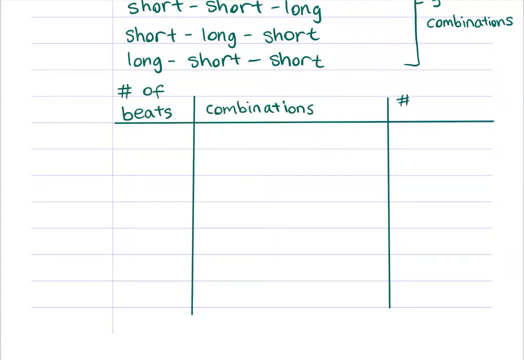 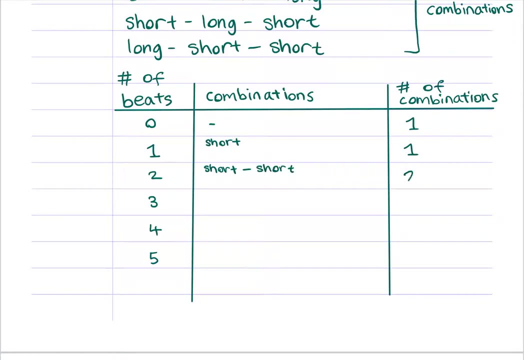 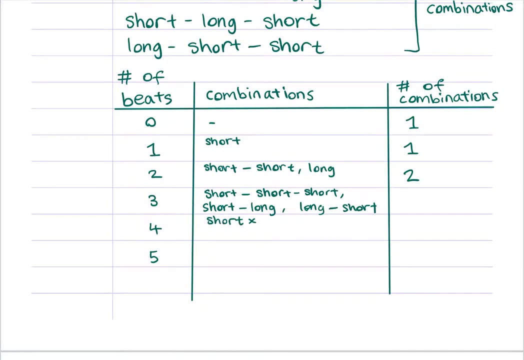 For a one beat rhythm, there's only one combination: one short. For a two beat rhythm, there are two combinations: two shorts or one long. For a three beat rhythm, there are three combinations: three shorts, one short and one long and one long and one short. We've already done the four beat rhythm, so 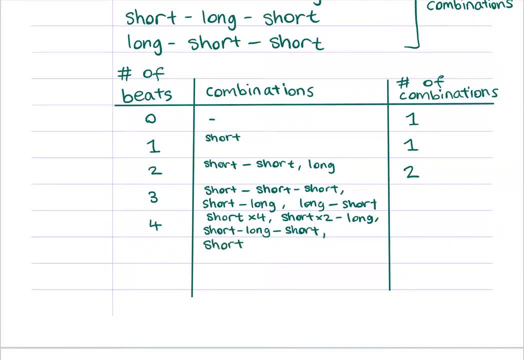 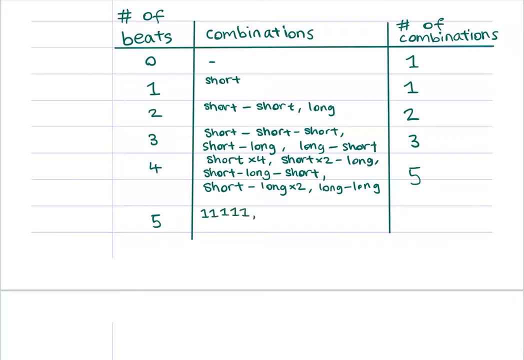 I'm just going to put this here. All the possible combinations are shown here. For the five beat rhythm we have eight combinations as shown here. Please note that a one represents a short and a two represents a long. By now most of you probably recognize this pattern: One, one, two, three, five, eight, thirteen. 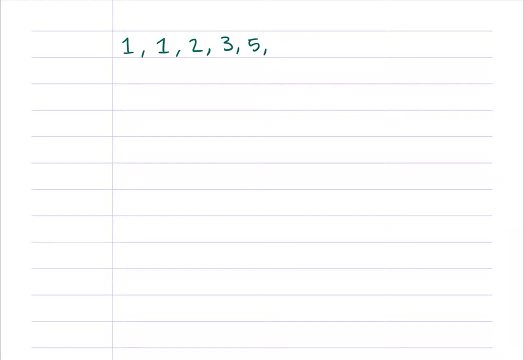 This is a hematschandra sequence discovered by the Indian poet and polymath Akarya Hemachandra around the year 1150 AD. Now it's more commonly known as hemaantra or hemat besch mari. But if somebody says, don't collect it, you can't hold this attraction and continue. That's exactly what we're going to do. 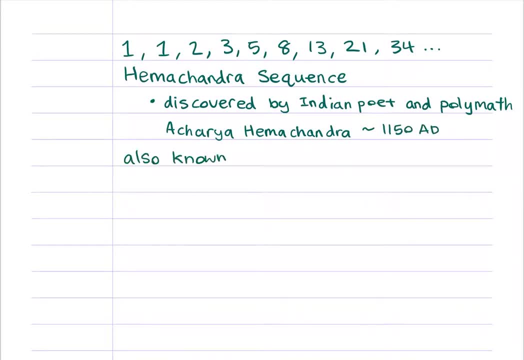 I hope you found a helpful этомat geschimme. Please remember to leave a like. If you're not, i'll at ten o'clock. as the Fibonacci sequence, after the Italian mathematician Leonardo of Pisa, also known as Fibonacci. However, knowledge of the sequence dates all the 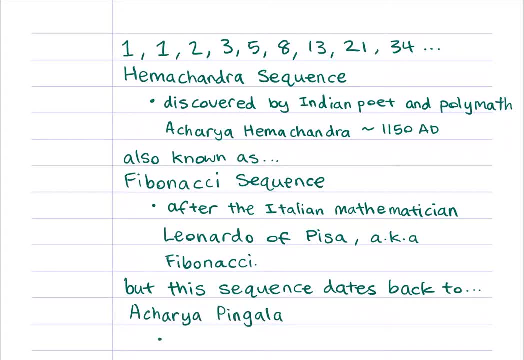 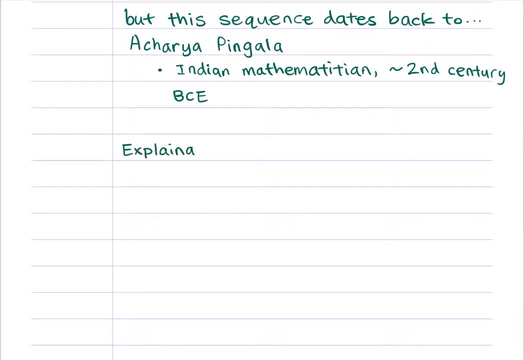 way back to the Indian mathematician Akarya Pingala in the 2nd century BCE. The hematangial sequence, or the Fibonacci sequence, is notorious for popping up everywhere we look For one. it turns up in Sanskrit poetry, of course. 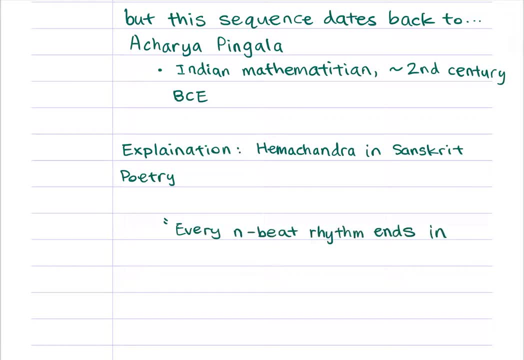 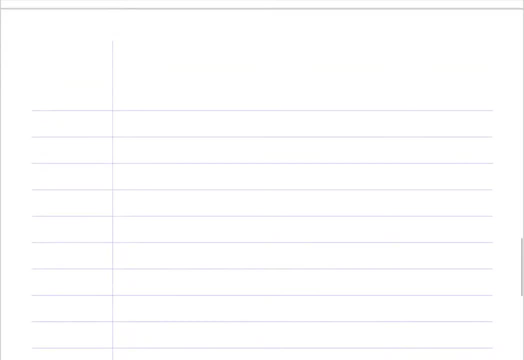 and Himachandra explained this in a very interesting manner. He simply stated that every n-beat rhythm ends in either a short or a long. just like that Done. But let's take a closer look at this: How many n-beat rhythms are there? 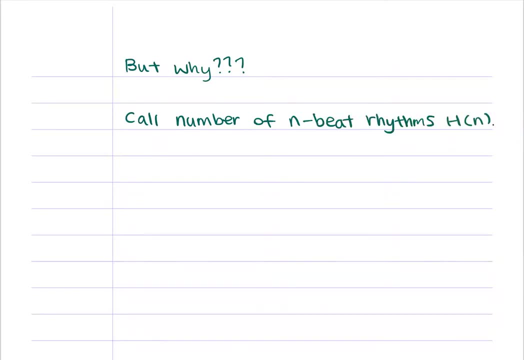 Let's call this h. If you have an n-beat rhythm that ends in a short, you have n-1 beats left to fill. So if you have n-1 beats left to fill, you have n-1 beats left to fill. 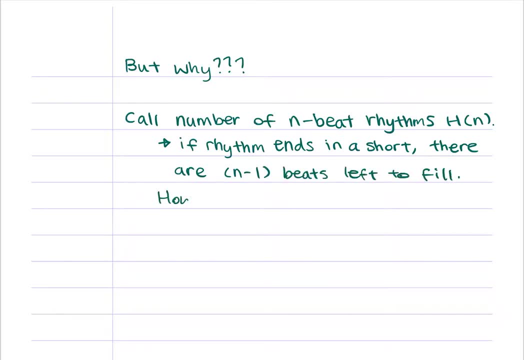 So if you have n-1 beats left to fill, you have n-1 beats left to fill. So how many n-beat rhythms end in a short? Well, it's just the number of n-1 beat rhythms, or h. If you have an n-beat rhythm that ends in a long, then you have n-2 beats left. 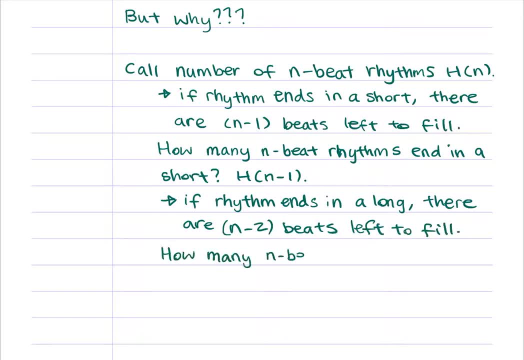 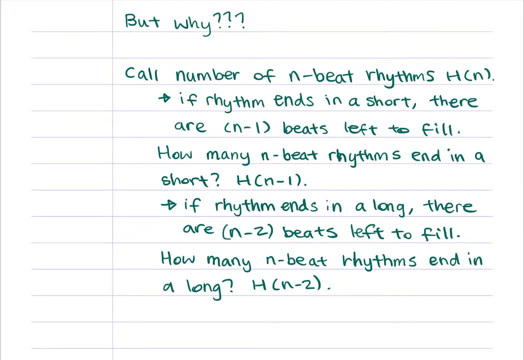 to fill. So how many n-beat rhythms end in a long Well, the number of n-2 beat rhythms, which is h, And from there we get that the number of n-beat rhythms h is equal to the sum of h and h. 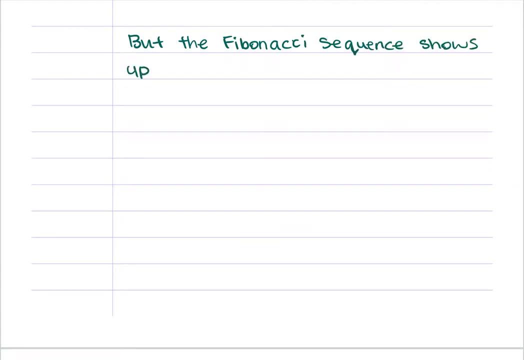 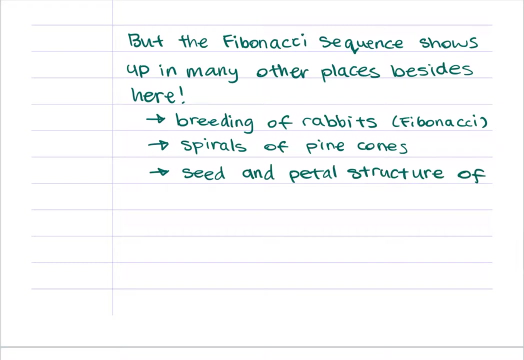 But this isn't the only application of the Fibonacci sequence. It also came up in the breeding of rabbits. That's actually how Fibonacci discovered it- in the spirals of pine cones and in the seed and petal structure of many flowers. Let's take a look at a beautiful 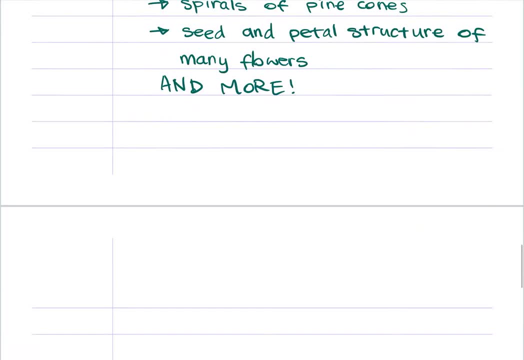 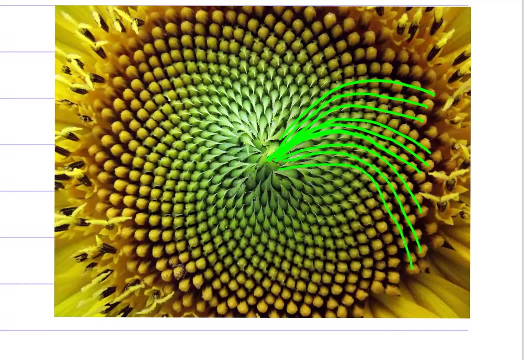 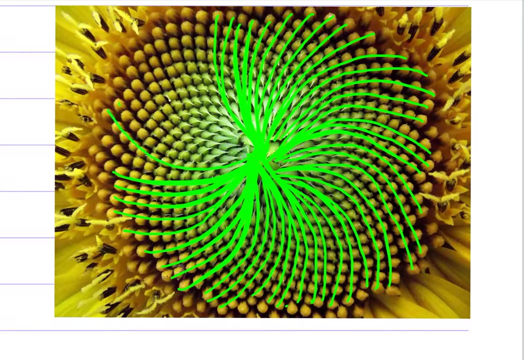 example, What you see here is the head of sunflower seeds. You can see the seeds positioned in a spiral. Interestingly enough, the seeds spiral in more than one direction, three, in fact, even though I only draw two, If you count the number of spirals twirling in opposite. 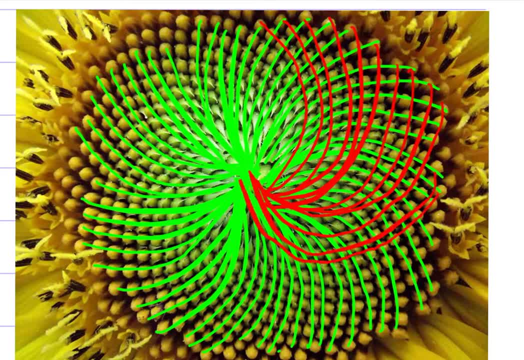 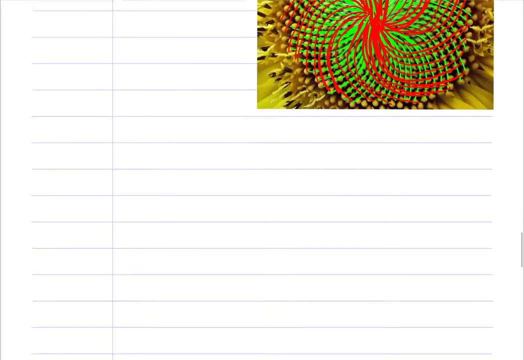 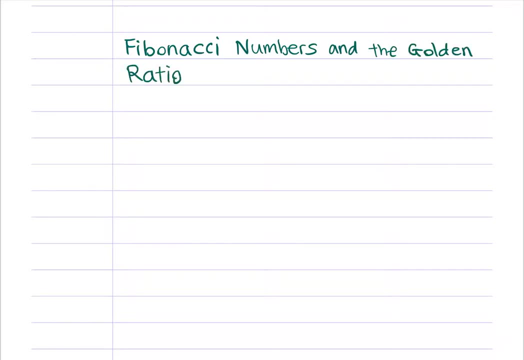 directions. the number of spirals are actually almost always two conductive Fibonacci numbers, which I find very interesting. Another really cool thing about Fibonacci numbers is that they are actually very similar to the golden ratio. So what's a golden ratio, you might ask? Well, two quantities are in the golden ratio if 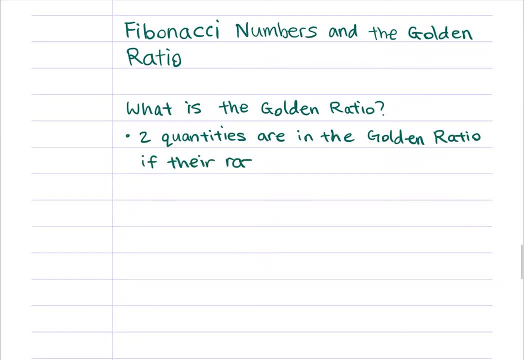 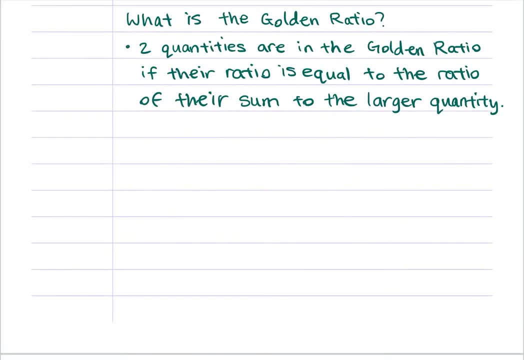 their ratio is equal to the ratio of their sum to the larger quantity. Now that sounded a little bit convoluted and confusing, so let me put it mathematically. Mathematically, for real numbers, a is greater than b, which is greater than 0. We have a plus b over a. 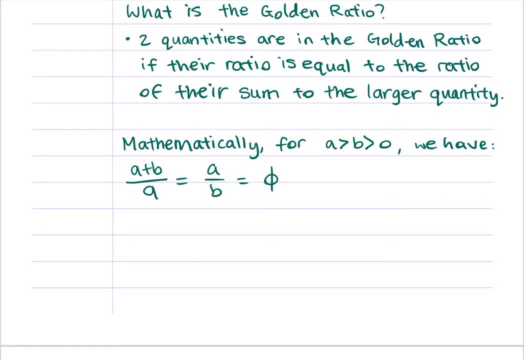 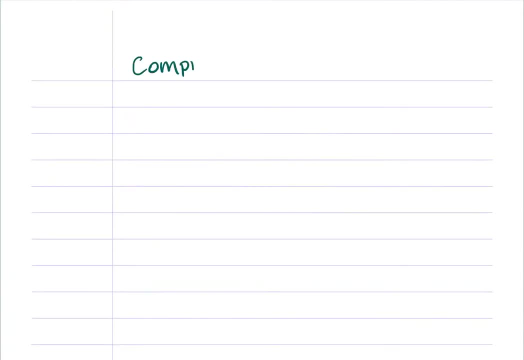 equals a over b, which equals phi. Here, phi is the golden ratio. Let's see if we can compute phi, shall we? So from the equation we just wrote down, I can substitute phi equals a over b into a over b. equals a plus b over a, to get 1 plus 1 over phi equals phi. Now, all we have to 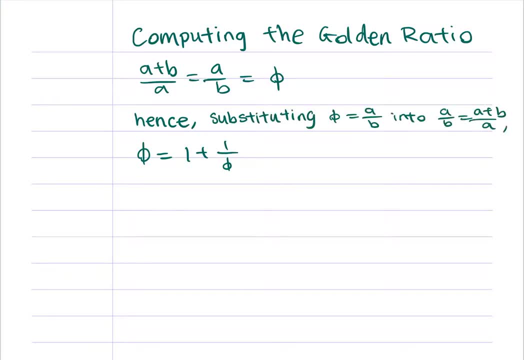 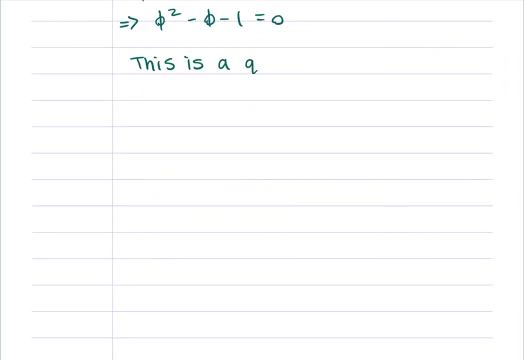 do is multiply both sides by phi and we get phi squared equals phi plus 1.. And then we can manipulate that solution. Let's do some more to get phi squared minus phi minus 1 equals 0.. And that's a quadratic equation which means it has two solutions. Phi equals 1 plus or minus square root of 5. 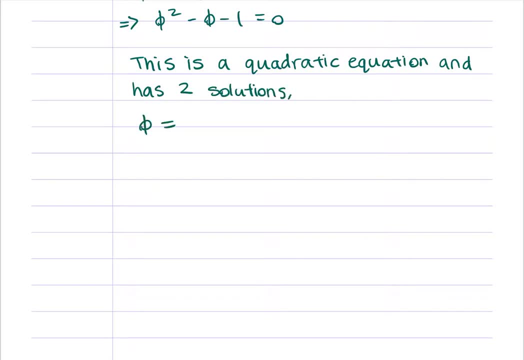 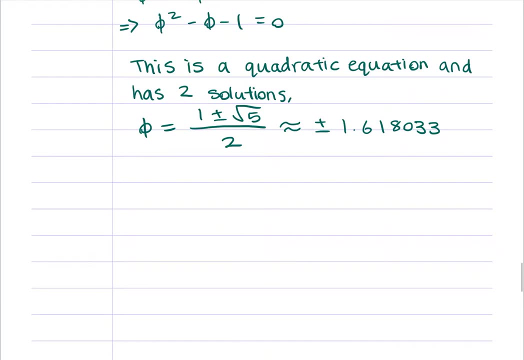 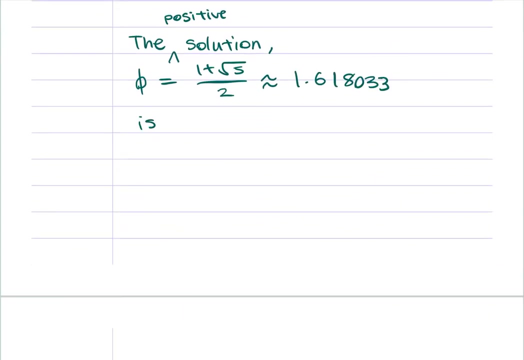 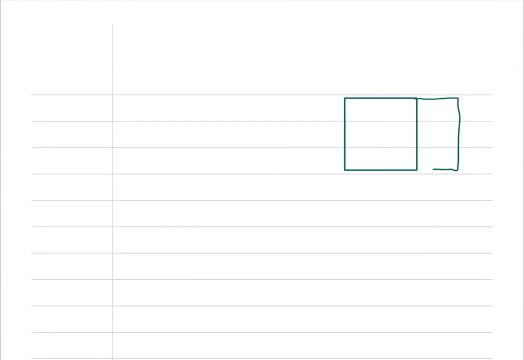 over 2, which is approximately equal to plus or minus 1.618033.. The solution phi is equal to 1 plus root 5 over 2, which is approximately equal to 1.618033.. Now the golden ratio has been of interest for a very long time due to the fact that 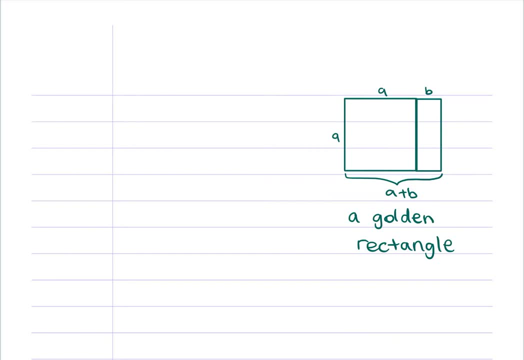 many believe that its proportions are aesthetically pleasing. Many artists and architects incorporate it into their work, usually in the form of a golden rectangle, a rectangle in which the ratio of a longer side to the shorter side is the golden ratio. Okay, 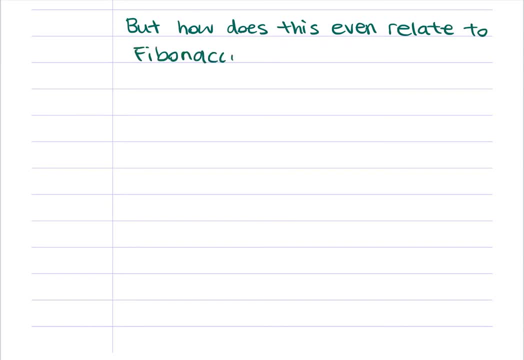 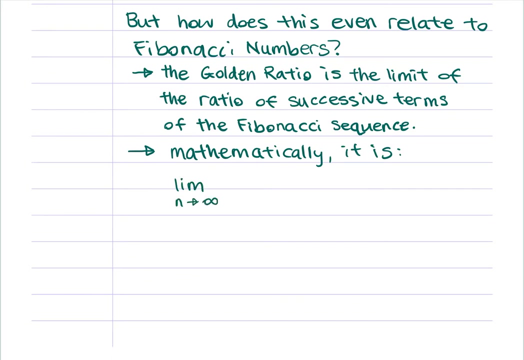 Okay, Okay, Okay, that's cool and all, but how does all of this even relate to the Fibonacci sequence? Well, the golden ratio actually is the limit of the ratios of successive terms of the Fibonacci sequence. To put it in mathematical terms, it's the limit of h over h, as n goes to infinity. 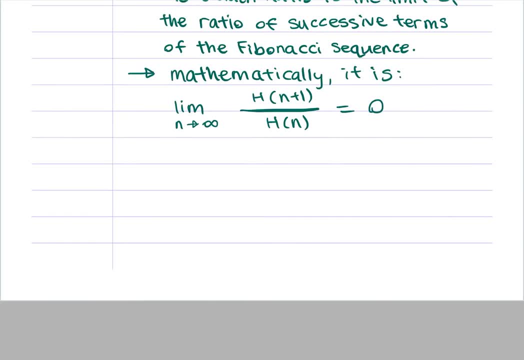 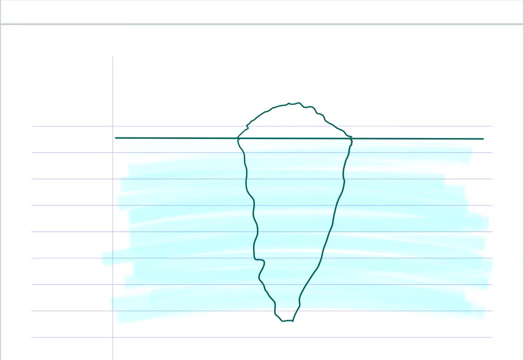 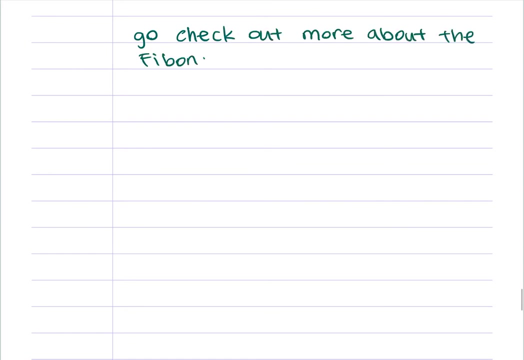 The Fibonacci sequence has been around for a very, very long time. In this video, I've only just grazed the tip of the iceberg. There are so many cool and amazing connections you can make with this sequence that you can and should go learn more about. 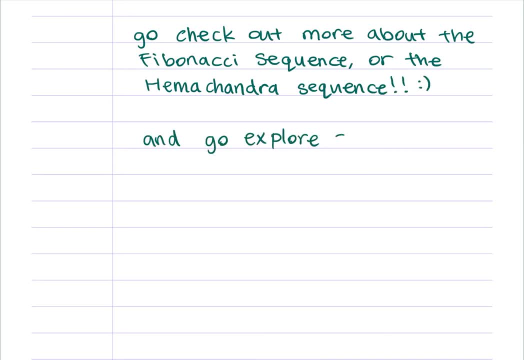 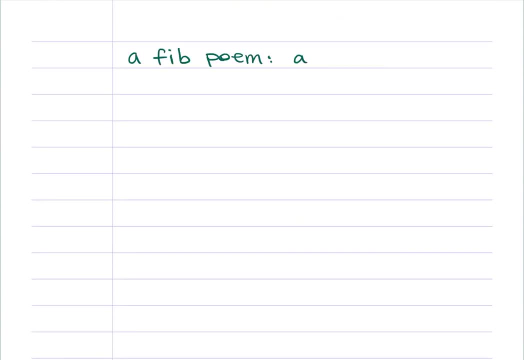 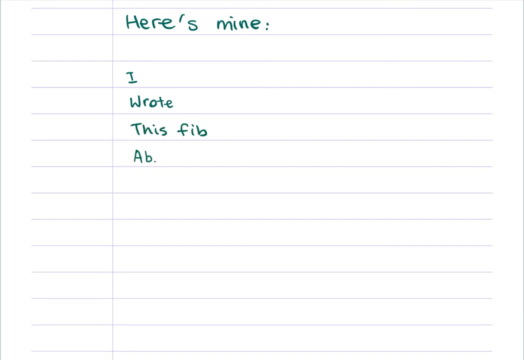 I hope this video inspires you to explore more math-y stuff. In parting I would like to leave you with a poem I wrote. Its syllable count follows the Fibonacci sequence. Such a poem is called a Fib. Here it goes. I wrote this Fib to tell you about cool numbers for 3 blue, 1 browns math challenge.